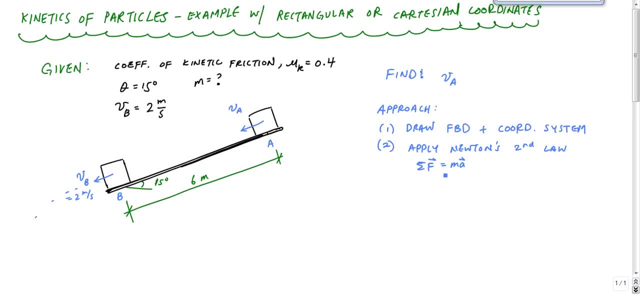 diagram parallels. you know this, this newton's second law. that's the way we want to do it, and then we're going to solve it, and then we're going to probably use some kinematics here. well, here let's go back a little bit. we're going to use newton's second law really to get 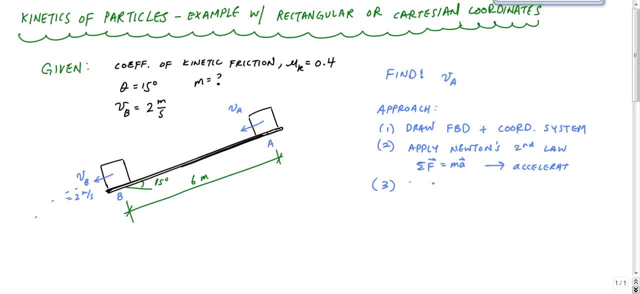 acceleration of the particles, acceleration. and once we have acceleration, what we want to do is apply kinematics- kinematics to get the velocity. okay, so let's see how that's done. okay, let's go for it. so the first thing that we want to do is let's draw a free body diagram of the box. 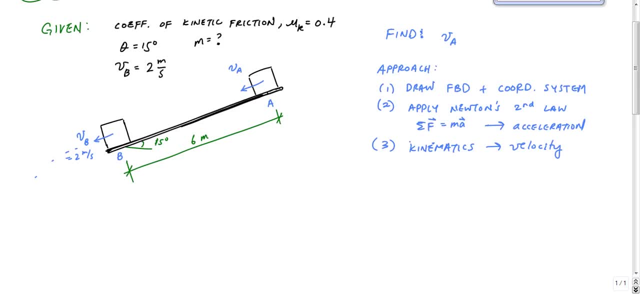 somewhere along this path here, so somewhere along this path here. so maybe i i'll draw the box over here. so if i, if i look at that box right here at that instant of time, so here one fbd or or schematic view, schematic here, schematic of my, of my particle and the forces that it experiences here. 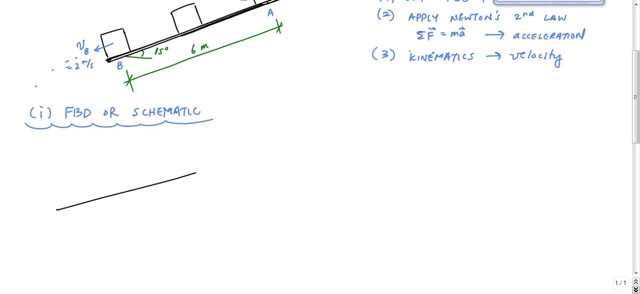 so i have this 15 degree incline. i have a box here like this, right here, and let's make sure it's a little bit cleaner drawing. let's use my straight edge. yes, okay, right here. and this angle right here, this angle of the incline is 15 degrees. what i wanted. 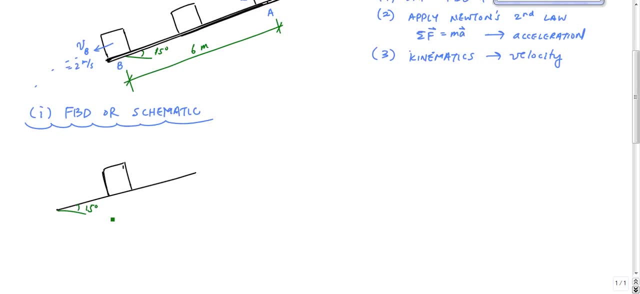 to do is i: i know that i'm going to need an external force diagram- okay, an external force diagram- and i want an inertial diagram. so i want this exact same drawing here. fortunately, i have like a computer kind of deal right here and i can just bam, paste it onto here and move it into place nice. 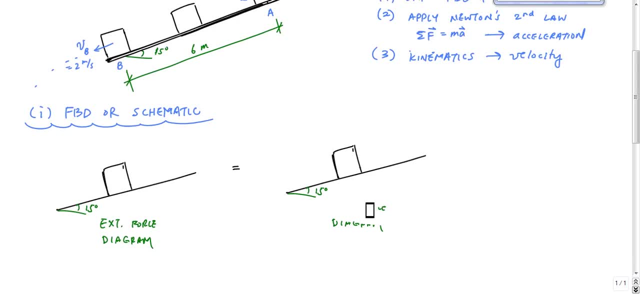 right there and i don't need this stuff right here. this, on this side of the equation, will be my inertial diagram. this i'm going to call the inertial- oops- inertial diagram. this will be my inertial diagram here, and and what we want to do- really the first thing when we draw this fbd- is establish what 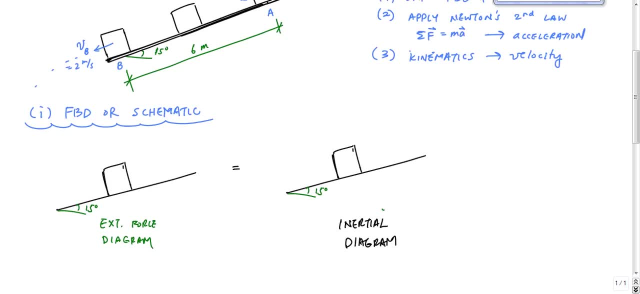 our coordinate system will be and because, you know, just for convenience sake, because i know my particles are moving down this path, i'm just, i'm just going to change the way that i'm going to choose, going down the path as my plus x direction and my plus y will be. 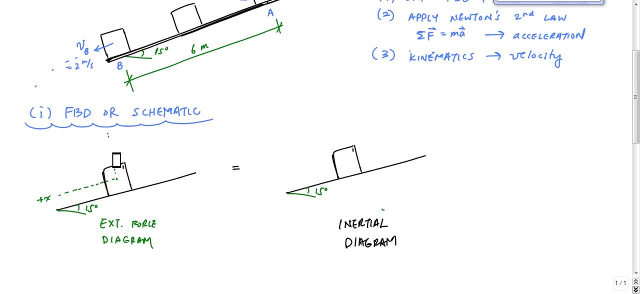 upwards, plus y here, bam, plus y. okay, like this, plus y will be that direction here. and then i want to do the same thing here. i want to say: uh, here, and really it's not really that we're drawing on the particle, it's more like, um, we have, we're establishing it over here. 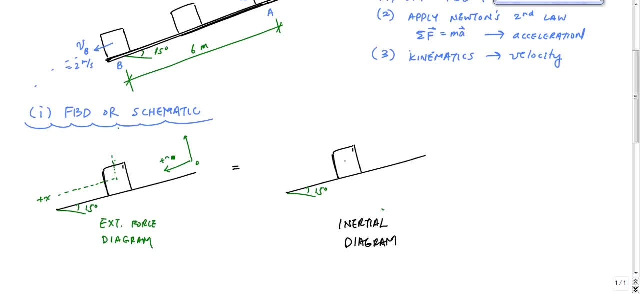 if this is my origin, as plus x and plus y, like this right here, and we're just putting it here, this, these dotted lines, just so that we can draw the forces better and come up with angles and things- okay, and the same thing here we have. we want to keep the same x and same y and what we'll. 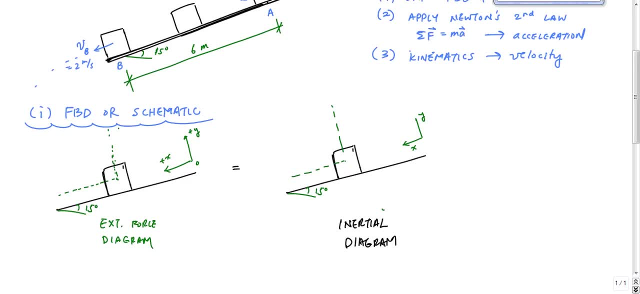 have is this: you know, this plus x direction and this plus y direction will be consistent on the particle. and so now i have here, let's start with the external forces i have here. i have a normal force on the block. okay, normal force on the. uh, i'll call it. 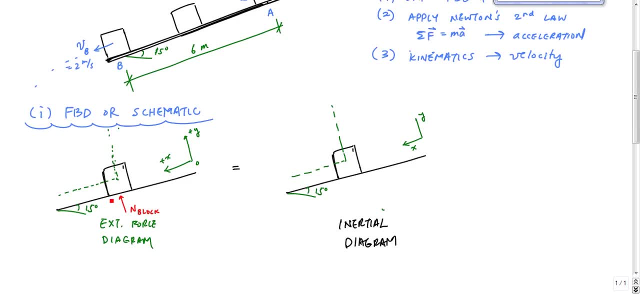 block, okay, and block here, and then i have the force of friction, f sub f, i have the weight of this block, so i'm going to go this straight down, w like that, and i don't think there's any other external forces. i think that's about it. okay, i think that's it. and then here the inertial side. 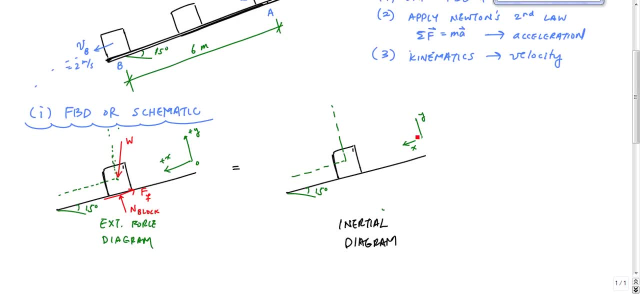 the inertial side. i just want to draw my inertial terms in the same direction, or draw them in my positive sense. you know, i don't know what the resultance of this is going to be, but i want, i'm just going to draw it in the positive. i'm always going to draw my m a x this way and m a y. 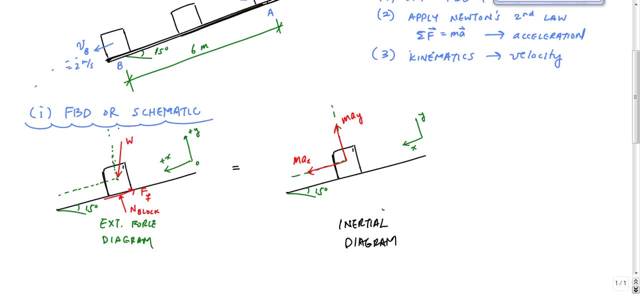 this way, right here, and some of you are practicing. why did you draw m a y? why did you draw m a y? well, i just drew it just to be complete, but the reality is that this block never moves in the y direction and the y is actually zero. okay, that's going to help us out a little bit later, all right, so this: 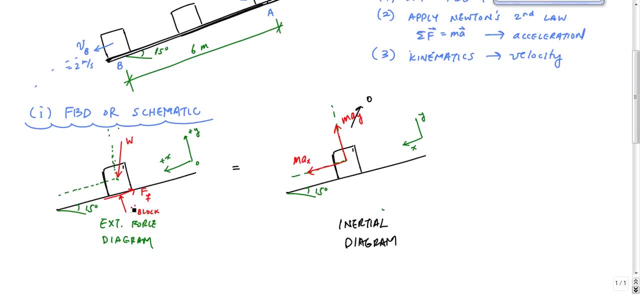 is our, our external force diagram and our inertial force diagram. we got to work out some geometry and what's something. you'll notice that this is 15 degrees and just by you know parallel lines and all that other stuff here. this is also 15 degrees and what we're going to do is break this up. this. 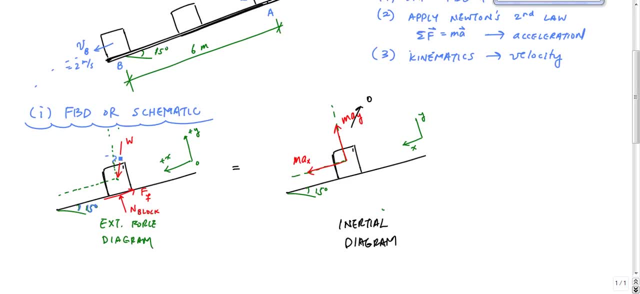 this weight is going to be breaking, broken up into, let me, 15 degrees right there. this weight here is broken up into the a, y, a y component and an x component. okay, so hopefully you can see that coming, but that's what we're going to be doing right here, and so now the next part. here once. 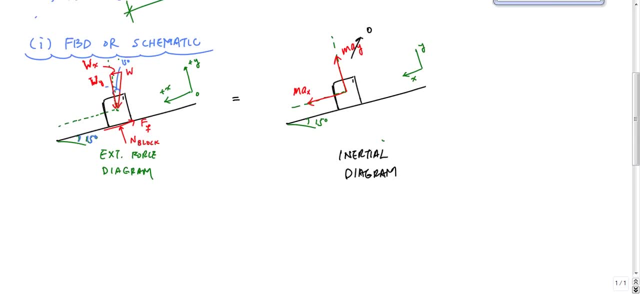 you have a good external force diagram and a good inertial force diagram. inertial diagram, then it's all about applying newton's second law or the equation of motion. okay, apply f equals m a. okay, apply f equals m a. right here. and so here, what we're going to do is because this f equals m. 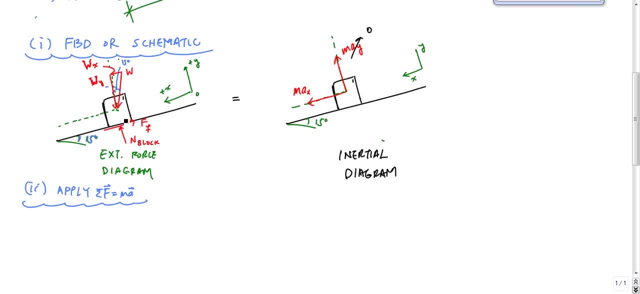 a is a vector equation. we're going to break it up into components and look at one dimension at a time. so in the x direction, some of the forces in the x equals m, a, x. my positive x is down, it's downwards this way, and so my equation here, by doing that, would be: i would have plus w, x. 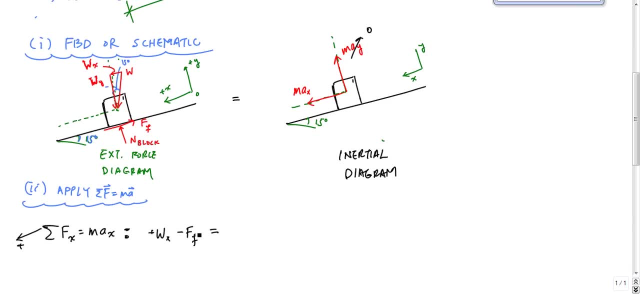 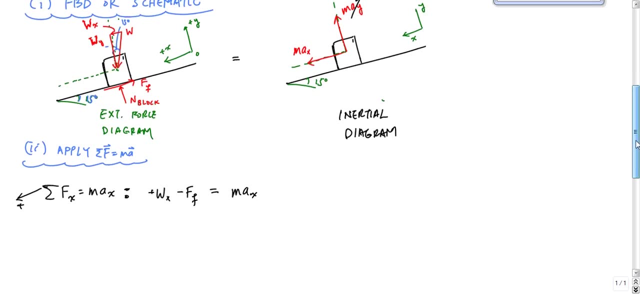 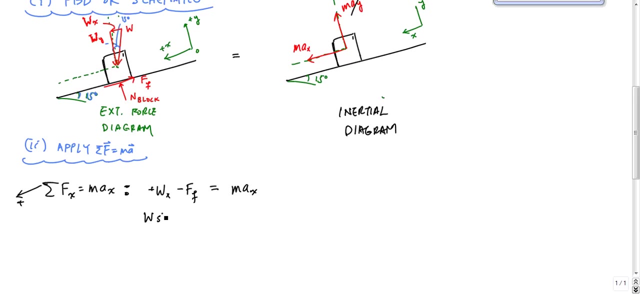 minus f of f is equal to. so here's my external force side is equal to m a x and just by pure geometry we know that w x right here. if i could, i could you know. normally i would just write this as w sine of theta minus f of f equals m a x. like that i would just run that, i wouldn't even mess. 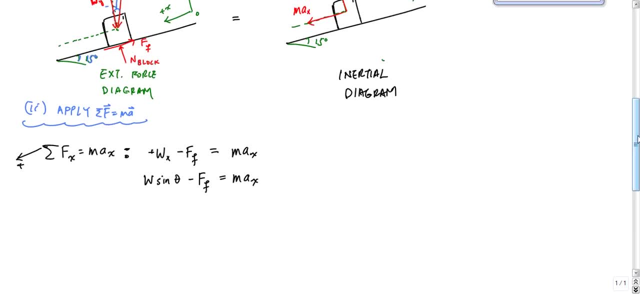 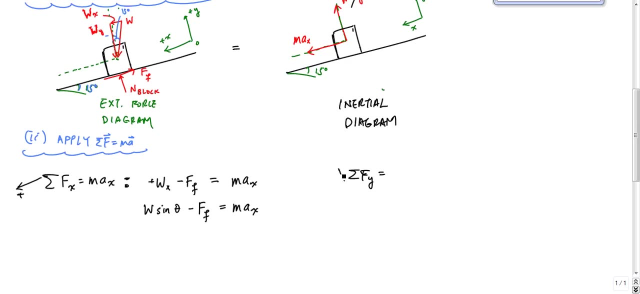 around with this w x business right here. okay then i want to do the sum of the forces in the y direction as well, some of the forces in the y equal to here. here's my positive y orientation, and this would be m, a, y right here. so i would have in the y direction, i'd have 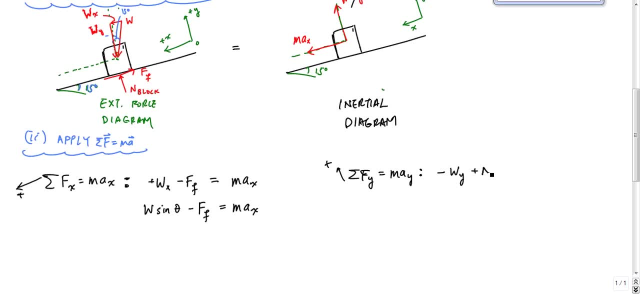 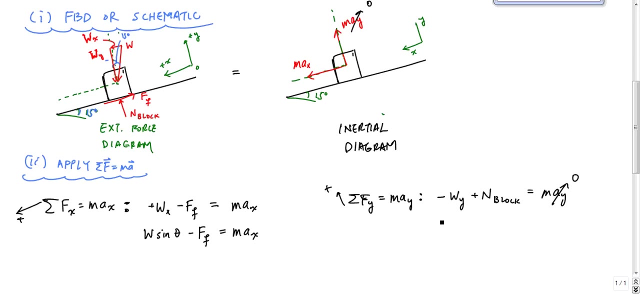 minus w y plus n, b, n block is equal to m a, y, which we already said is zero, because our, our block never moves in the y directions here, and that just tells us that this w, and then again, uh, again, i wouldn't normally write this w? y, but this would be minus. 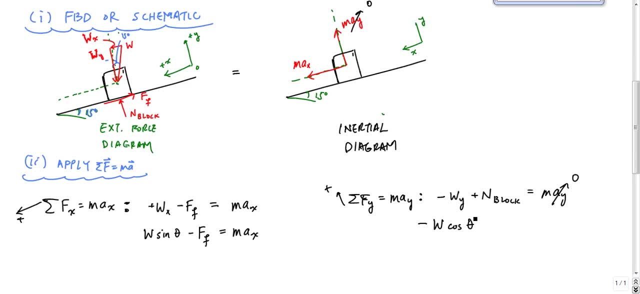 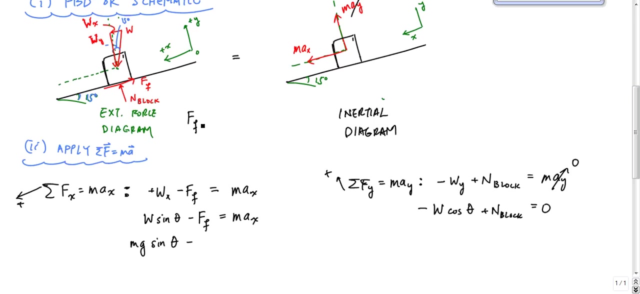 w, cosine of theta, where theta is 15 degrees plus and block is equal to zero. okay, so that's, that's good news. so what? what you see here is you you'll see that this w really is unknown. this is mg sine theta minus, and if you recall the definition of the force of friction, f of f, right here it's gonna be. 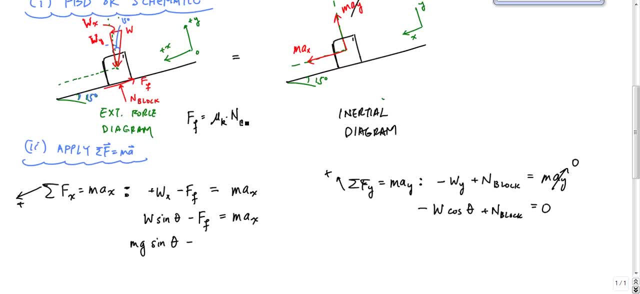 kinetic mu k times the normal force right here. okay, so the coefficient times the normal force on the block right there, and this is this other equation to help us get rid of an unknown. so this right here is this: mu k times n block here is equal to m a x, and so what we have in this equation, 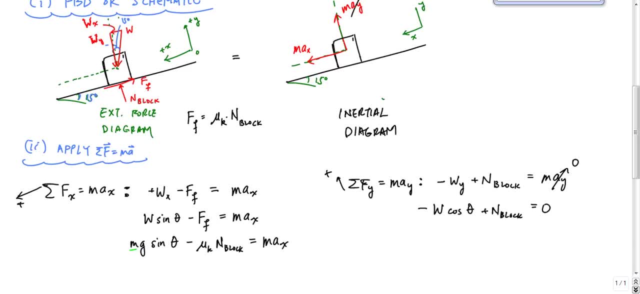 here is, we have one, uh, two and three unknown. so here i'll circle this one, i'll put a block around this one, because it's a block, and then here i'll have- oh, you know, that makes it look like: well, actually the mass is also unknown. but here, bam, i'll do this right here, and then i gotta. 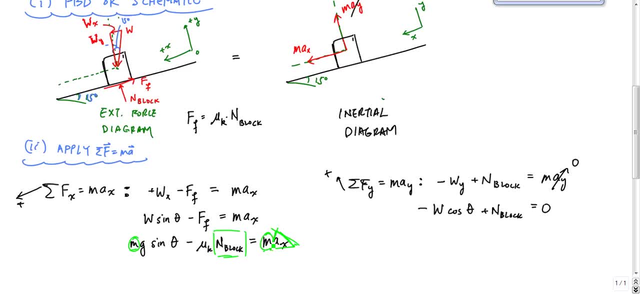 circle the mass there. so really i have one, two, three unknowns and and really only two equations left. so let's proceed with the way it is. i'm sure some of you can already see what's going to happen here. so i have this: minus mg cosine theta plus n block equal to 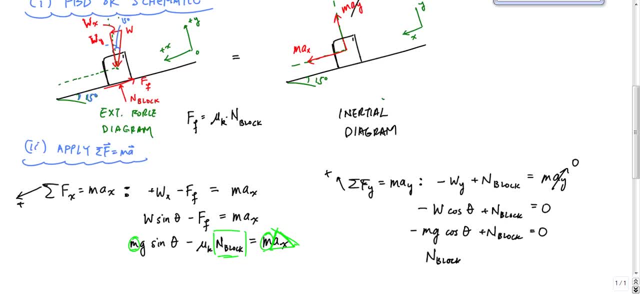 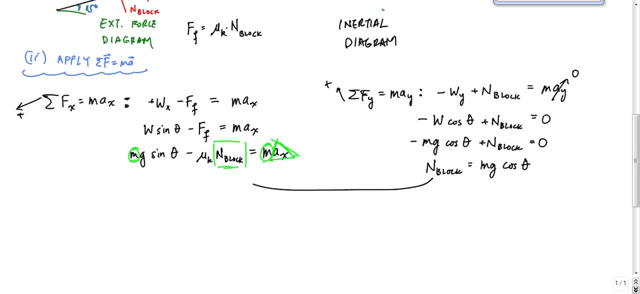 zero, and here n block is equal to mg cosine of theta, right here. and so now i'm going to substitute this into here, i'm going to combine those two equations right here, and so that'll just be mg sine theta minus mu k. mg cosine theta is equal to m a x, and what i have here 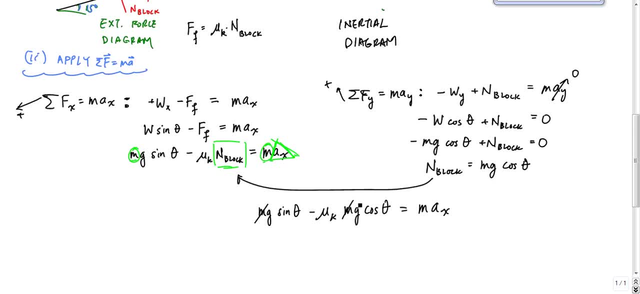 look at that, look at how that works out. it's that these masses all cancel out right here, and that actually happens a lot in, uh, in dynamics problems, especially when the mass isn't given, you know, the masses usually will cancel out and and here what? what this will become is, you know, quite simply, this is there's only one unknown. 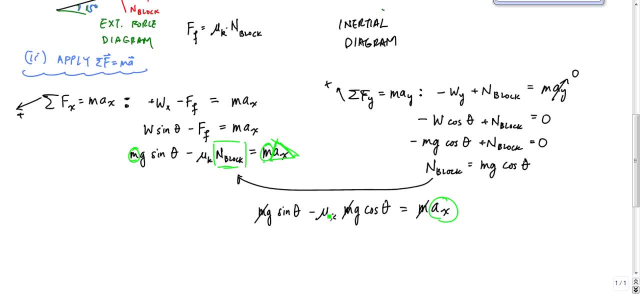 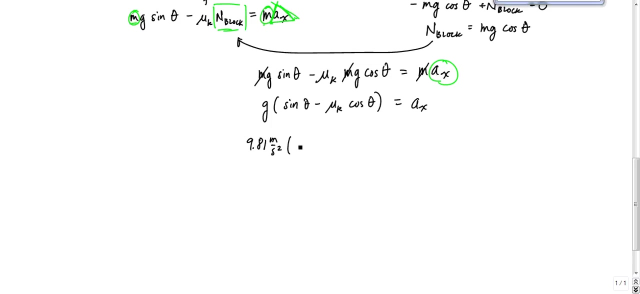 left here. it's this, this acceleration here, and what this gives us is that i have here g times the sine of theta minus mu k cosine of theta is equal to the acceleration in the x direction, and this acceleration, and if i now plug and chug some numbers, this will be 9.81 meters per second, squared times a sine of. 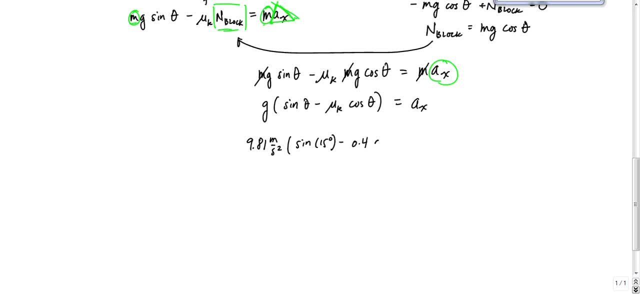 15 degrees minus 0.4 times the cosine of 15 degrees, and let me make that that bracket is equal to the acceleration of the x. this acceleration in the x comes out to ax is minus minus 1.25 meters per second squared. and what this? 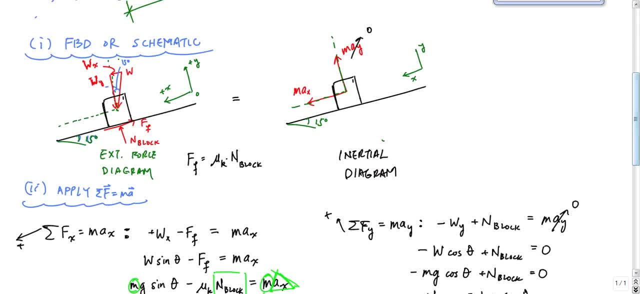 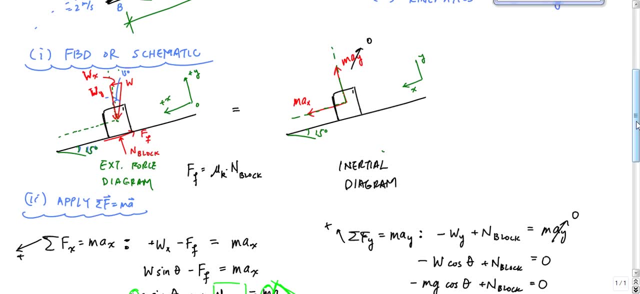 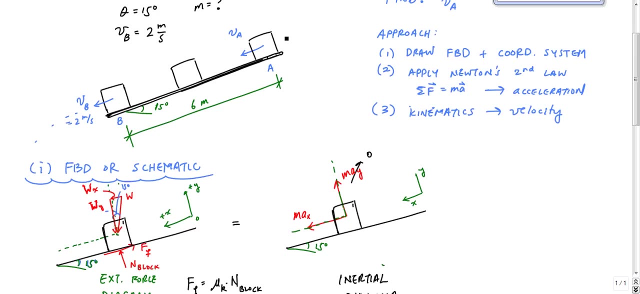 negative means is that the acceleration vector, or this inertial term, the acceleration vector- is actually pointing the other way. so this particle going from part, from point A to point B, is actually decelerating due to friction, right? so here. so with that, that acceleration is a deceleration, okay, so 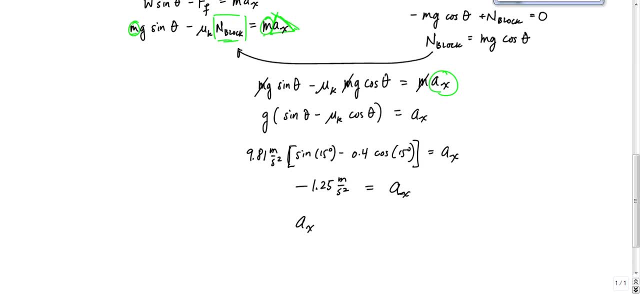 this ax is actually- if I want to write this properly in vector form- is 1.25 meters per second, squared this direction at 15 degrees. so an acceleration is provided as long as you give a magnitude and a direction that is your. that's your correct answer for acceleration, but that's not where we want to be. we also. 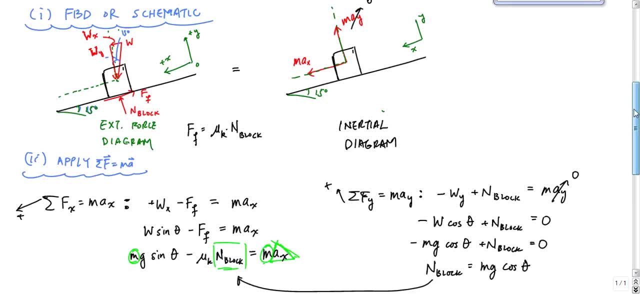 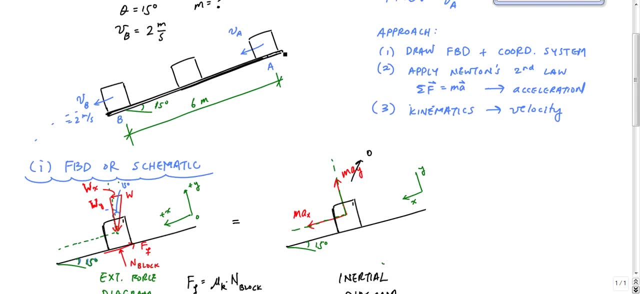 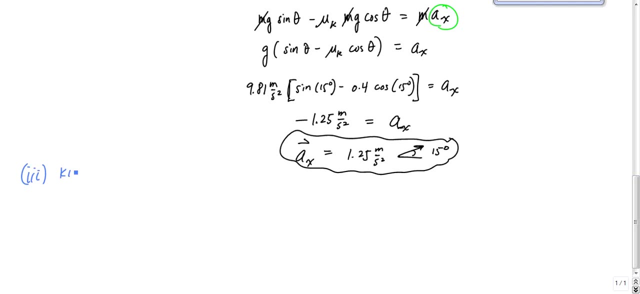 want to determine what the. now we want to use our kinematics and determine what the velocity of this thing is when it reaches, or what it was at point A. okay, and so here our last part of this is to use our kinematic relationships. two, three kinematics. and here I had just have plain 1d motion, and because the 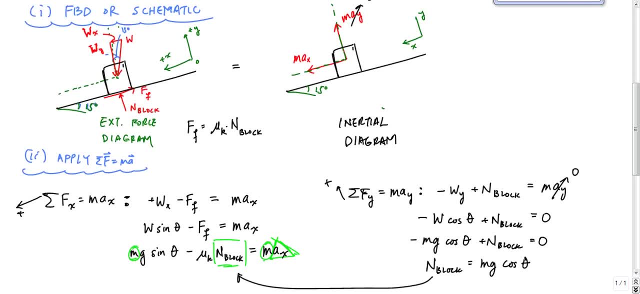 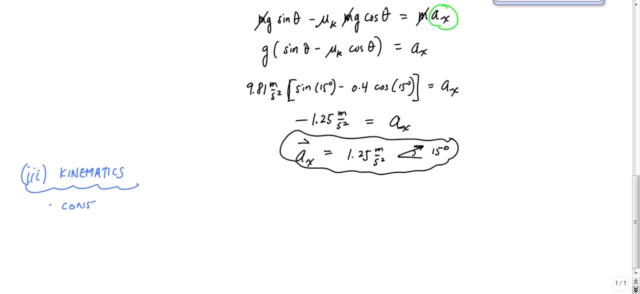 only thing that's really acting, the only force that's that's contributing to acceleration, if you will, is the, its gravity itself. I know that the acceleration is constant, so this is actually a case of constant acceleration. I don't have any sort of varying force to vary the acceleration. I 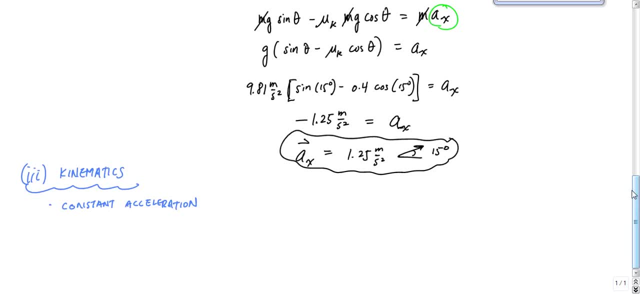 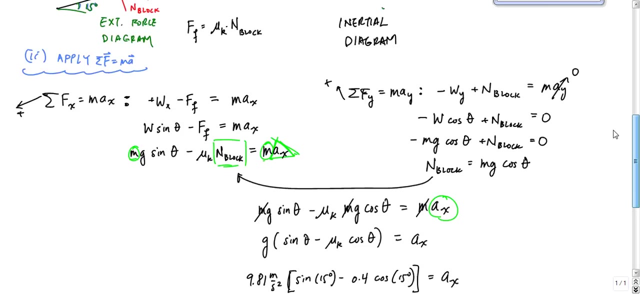 just all have a constant force, weight basically pushing down, causing it to move downwards. so here I have this constant acceleration case here, and that means, and what I also have in this case is I have the distance that this thing travels. the particle travels a distance of six. 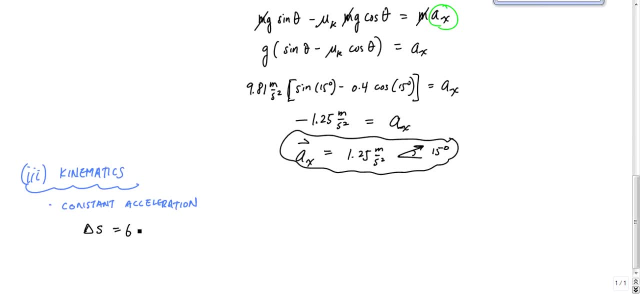 meters, six meters here, and I also have the. you know I have a final velocity VB which is here of two meters per second, squared right here, I'm sorry, two meters per second, this final velocity of two meters per second. so if you look through your constant acceleration equations and you know, I think, 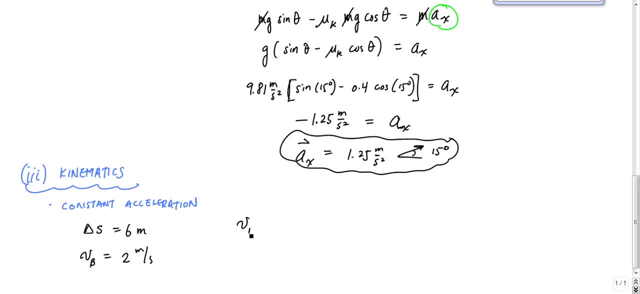 I should've worried about this. I'm sure I have a derivation of this somewhere, but here this you would use as VB squared minus VA squared is equal to 2 times the acceleration and the X times the change in position. right here, okay, this is just from that, really, you know, coming up with the costs and acceleration, it's you know. 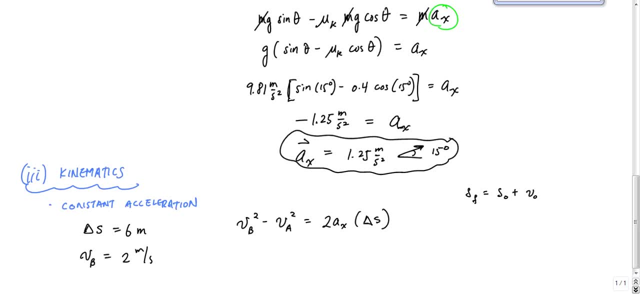 is equal to s zero plus v zero t plus one half a t squared, and then you had a velocity equation. velocity final is equal to v zero plus a t. if you combine these two equations and get rid of time, you get this. okay, that's what you get. and delta s right here. delta s is just s f s final minus s. 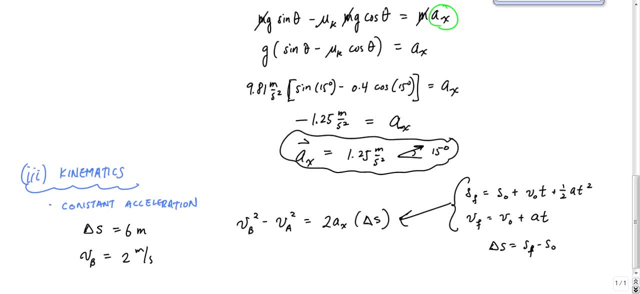 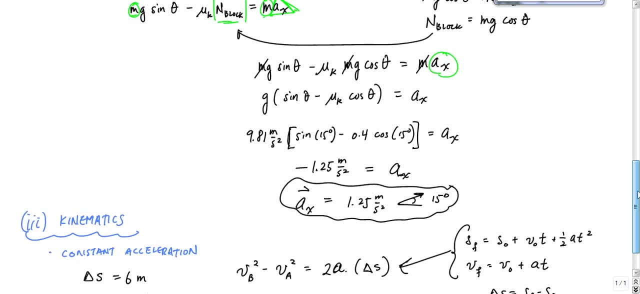 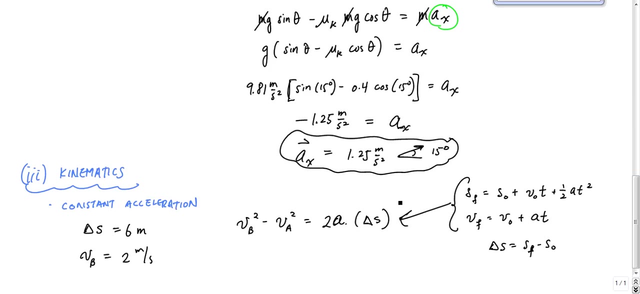 zero, okay. so that's what's going to happen here and that's where this comes from. or a acceleration in one dimension, or x in this case, right here, now, if we're going to keep this positive motion downwards here, okay, and our acceleration is in the opposite. so in this case, here, when we 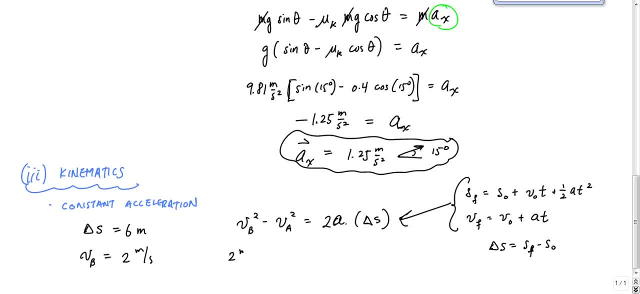 apply this right here: this v b squared, this is going to be two meters per second. quantity squared minus v a squared, the value we're looking for is equal to two times negative one point two: five meters per second squared. so this negative is really important because we're